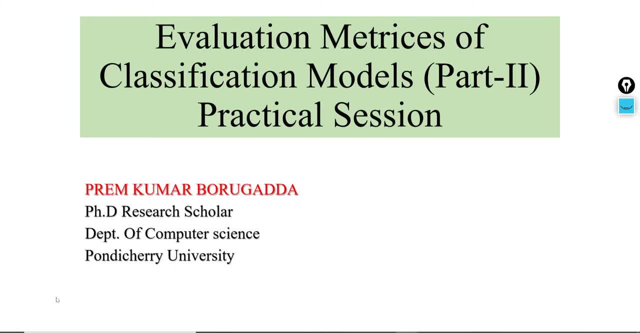 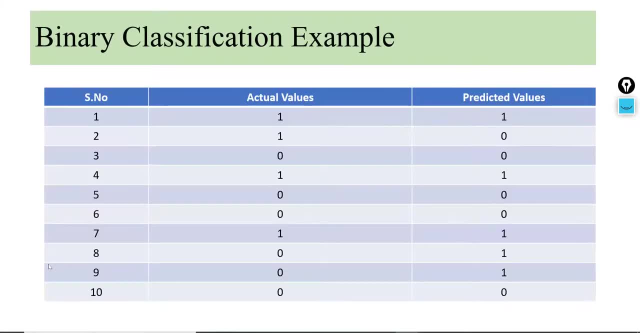 f1 score. so in this section we have to discuss about the practical section only. so if you see this, this is the binary classification example. so in the binary classification example we are taking the two values. so that is nothing but the actual values. so this is the actual values means. 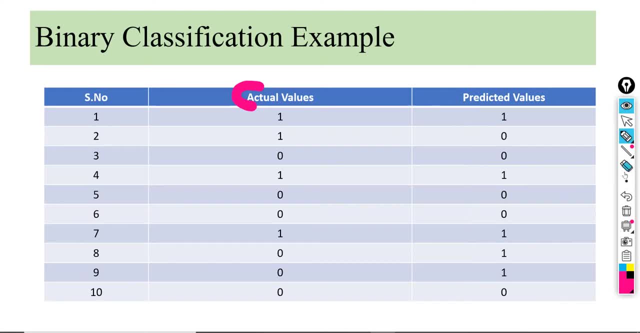 sorry. so this is the actual values. so actual values means this is our data set. in this our data set we have to x and y, x and y, so the y, this is the input variables. so so many parameters are there. so here our y value is nothing but the our target variable target. 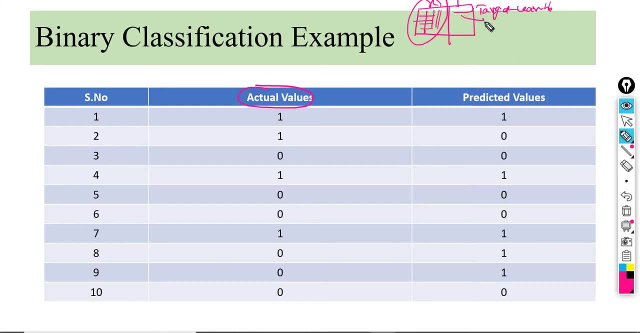 variable, so target variable: nothing but this is the our y y, true, so this is nothing but the our y values and this values given by the model. so in this actual values we have to consider in the 10 instances means 10 rows for this example. so in 10 rows we have the 10 values. 1 such zeros means this is the binary class, means only class 1. 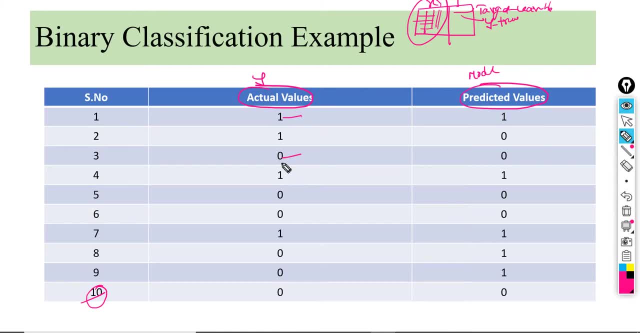 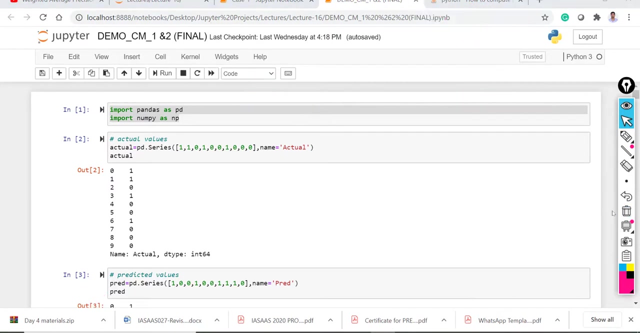 class 0. two classes are repeated, so this is the binary class. so based on these values- actual values and predicted values- we have to implement here on the confusion matrix. so first we have to import the required libraries, so that is nothing but the pandas and libraries. next we have to consider the actual values and this is the actual values and this is. 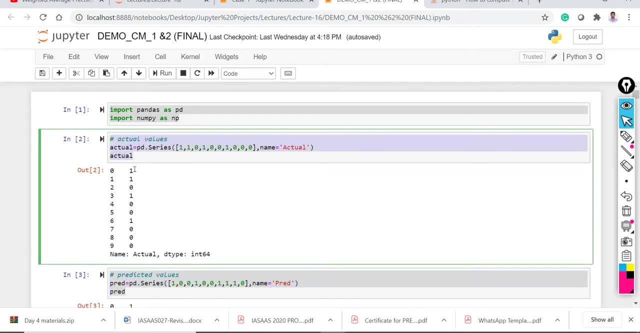 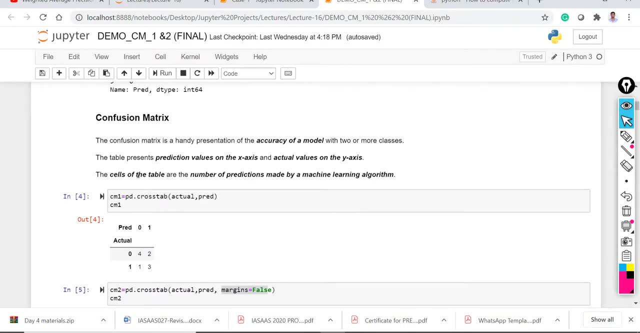 the predicted values. with the help of the pandas library, we have to considering the actual values and predicted values. so next we have to build the confusion matrix. so what is the confusion matrix? so confusion matrix, it is a handy presentation of actual, of model with two or more classes. 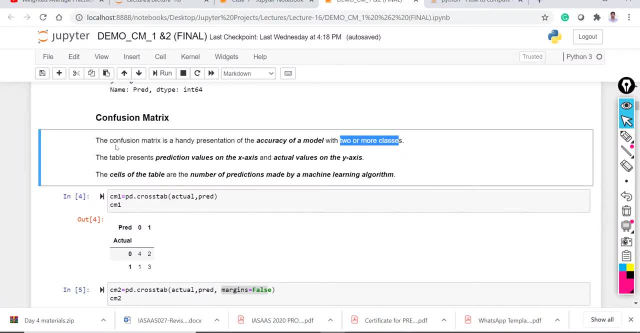 so in our event data set in the target variable we have the. if we have two classes, we have to use the binary class. if we have more than two classes we have to consider it is a multi class. so even it is binary class or multi class. so for accuracy of the model, with more 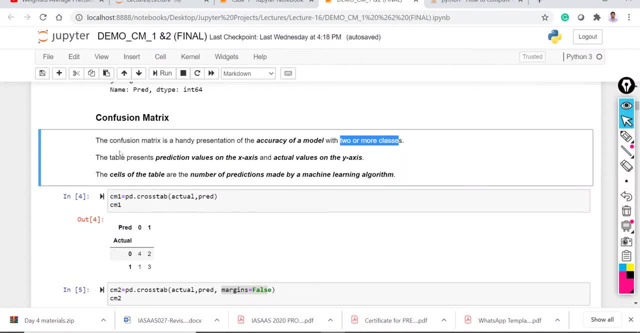 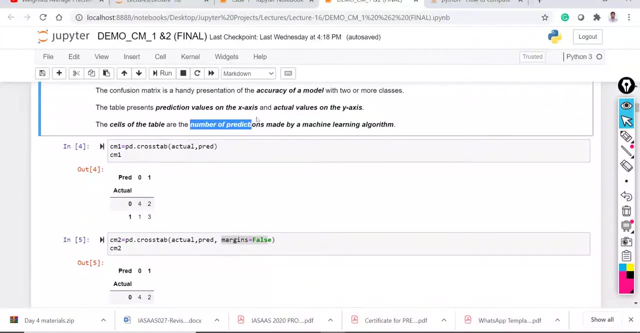 than two or two classes, and more than two classes we have to under the confusion matrix. so confusion matrix is a table presents the prediction values on x-axis and actual values on the y-axis. so the cell of the table are the number of predictions made by the model. model is nothing. 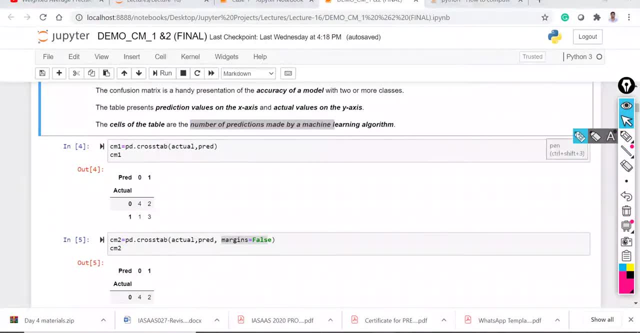 but the machine learning model. so here, if you execute this cell confusion matrix, pandas, with a pandas library using the method cross step, this is our actual values and this is predicted value in this values. so predicted values on the x axis. so this predicted values i am considering on x. 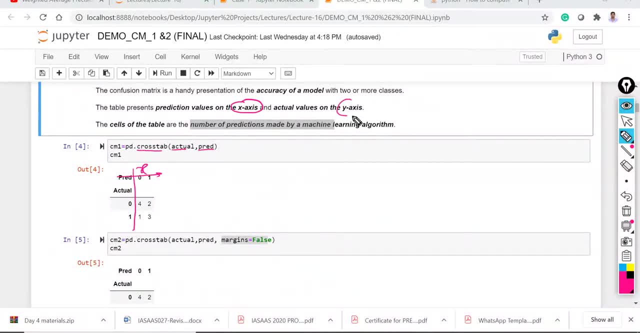 axis and the actual values we have to consider in y axis. so this is the our y axis. so means: so this is our confusion matrix. in the confusion matrix, this is the 0, 1, 0, 1- so this is the y axis- is nothing but the actual values, and this is nothing but the x axis- predicted values. so this is the. 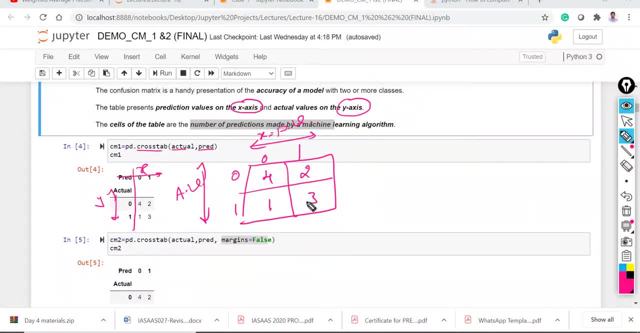 value 4, this value 2, this value 1, this value 3 means here this value i am considering as the true negative means: this is the negative, 0 is the negative. i am assuming, like that 0 is negative and positive is 1, so here 0 is equal to negative and positive is equal to 1. 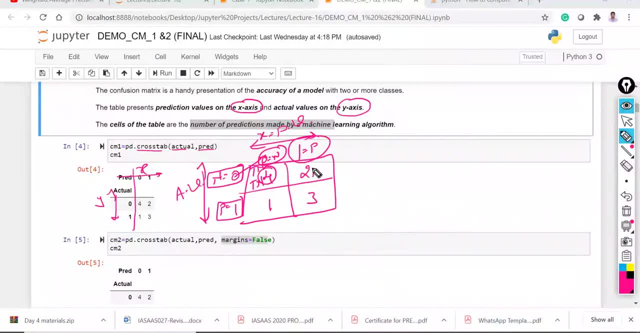 so means 0: 0. both are matching. this is the true negative, this is the false positive. this is the true positive and this is the false negative means our tn value 4, fe value 2, fn value 1 and tp value 3. so this is the confusion matrix. so here: 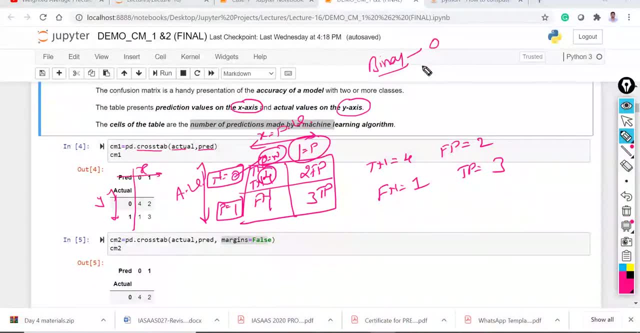 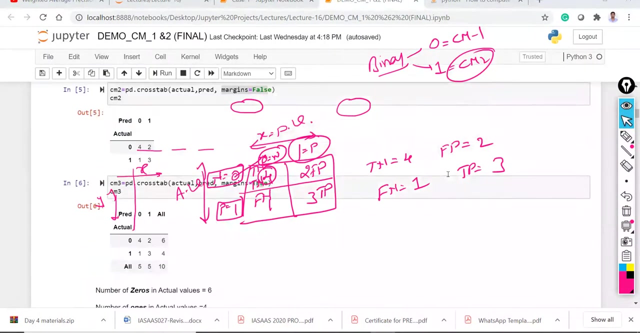 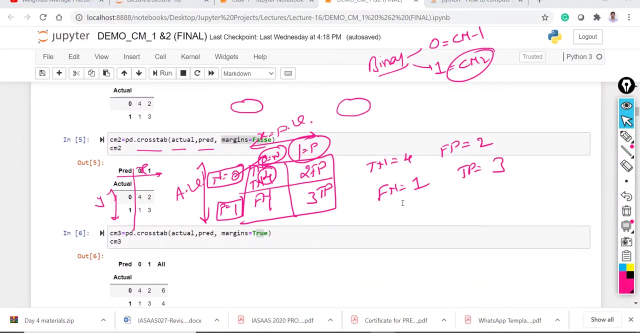 binary class. binary class, there are the two classes, class 0 and class 1. for class 0: 1 confusion matrix- confusion matrix 1. and class 1- confusion matrix 2, like that. so this is one confusion matrix because the method f1 is the usual 1 and f2 is 계속 and here the working어요. 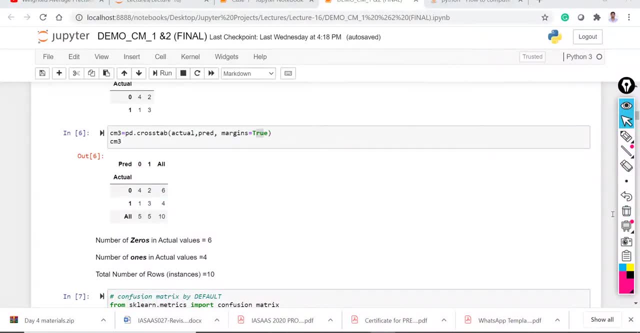 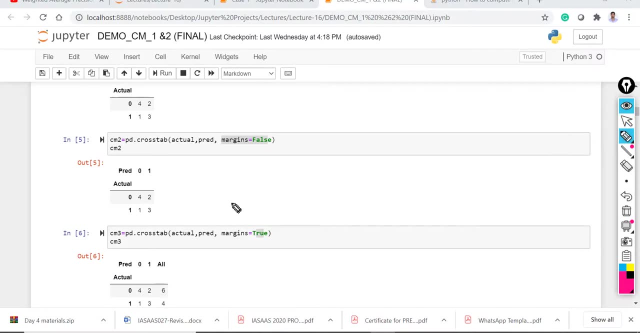 is very easy for us. so let's take the tree of��: so if maximum, Then condition f1 means that f2 is positive, when i always start by: is equal to false. margin is equal to false means it comes there in only confusion matrix when a margin is equal to true. so this is the statement. so when 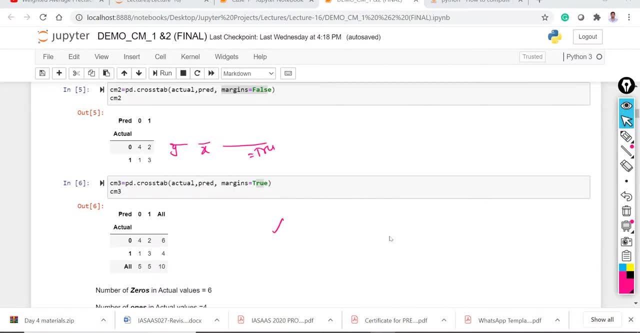 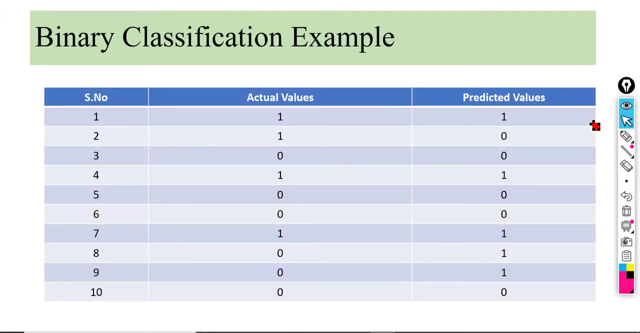 margin is true means it will calculate the sum of the values, sum of the various means here, number of zeros for total six and number of one four means in our data set. so this is our data set. if this is our data set, if you see how many number. 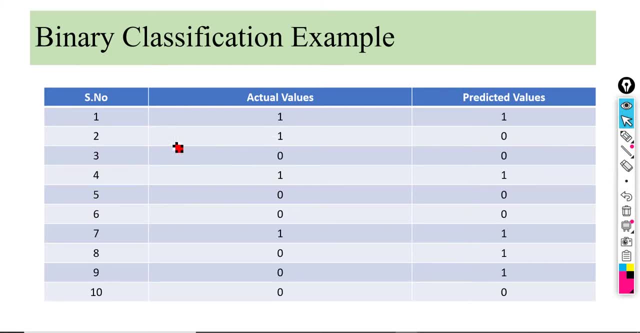 of ones here one, one ones and zeros. so here one means one, two, three, four, so number of ones. for number of zeros: one, two, three, four, five, six, four, five, six. so number of zeros: six. total: ten instances, total, ten instance. so here number of ones: four. so 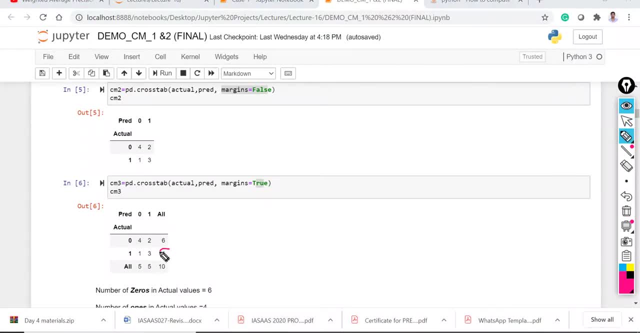 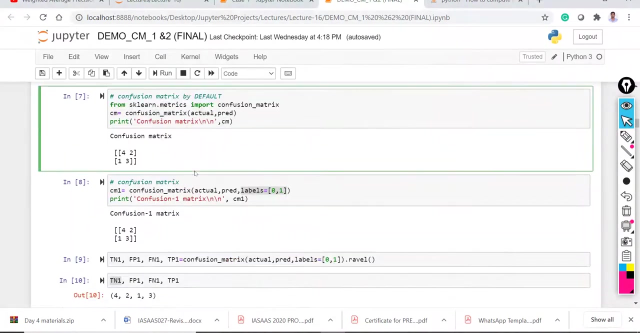 number of ones. four means, see here number of ones, for in actual values a number of zeros is six, total ten and predicted values number of zeros is five and number of ones is five. so this is the confusion. matrix cell number seven. so if you see, observe this. 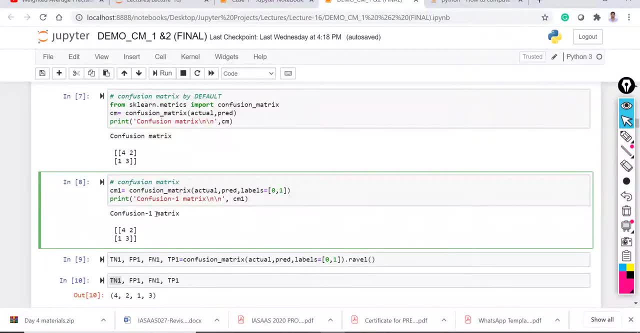 cell number seven and cell number eight, so coding little bit different, but the output is same. here the confusion matrix is applied on the actual and predicted. but here actual, predicted and labels is equal to zero comma one, so label equal to zero comma one. so here both are the same confusion matrix. 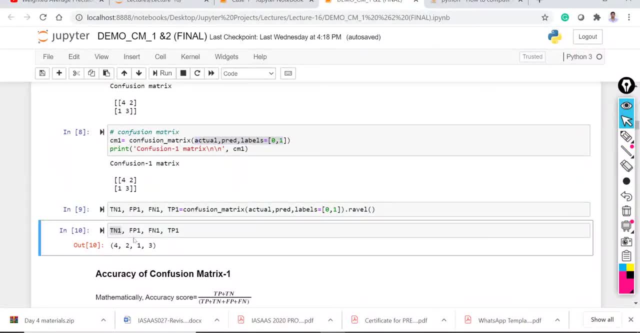 so from this confusion matrix we have to getting the values four comma two. so in this confusion matrix here, this value true, negative, false positive, true positive and negative. so this value true, negative is four, this value will be four. and if we will be two and this value one and this value three, so if you six and 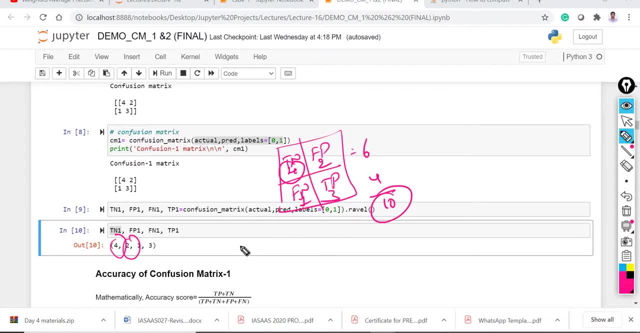 this is four, total tens, ten instances. so here means number of zeros is equal six, number of ones is equal to four. actually this is negative and this is positive, actually suppose so total number of zeros is six, but predicted number of zeros is five. actually number of ones is four, but predicted the number of ones is equal to five. means: 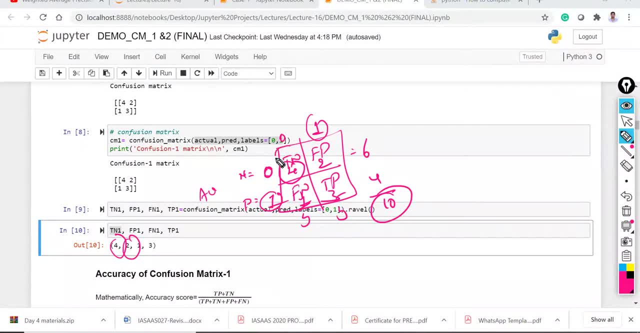 it is somewhat wrongly predictions. so here the diagonal elements, true positives and true negatives, this is the correctly predicted by the model, correctly predicted by the model, by the method. in this one, both variables we could get, is seems herself, вер chicks, and this diagonals. the diagonals means FB and FN are the wrongly predictions. 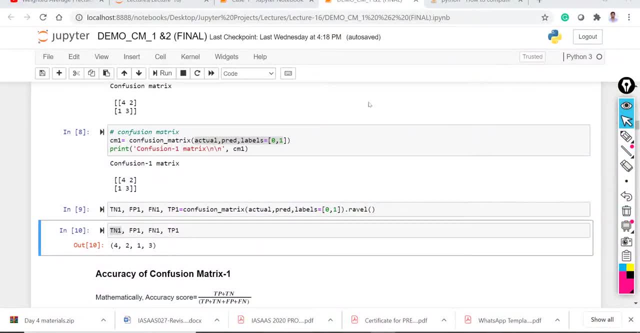 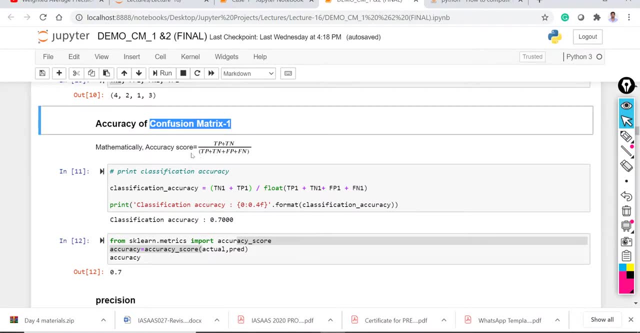 Pratik, brooder glee predictions by model. so if you see the accuracy of the confusion matrix one, It is got same naming after the number of zeros. so confusion matrix one It is the factories where we are considering the worth. wrong there is entire structure, the third is called half divided by two. that is because it is notام but the file type of the world. in this case, if you change the value, then one is less than勉 y and this was hidden in the teu Moscow method. but if you take another case can be. 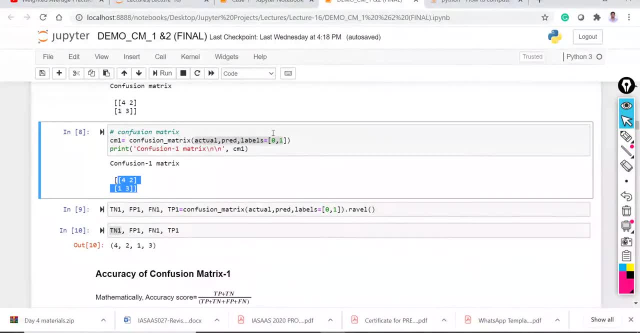 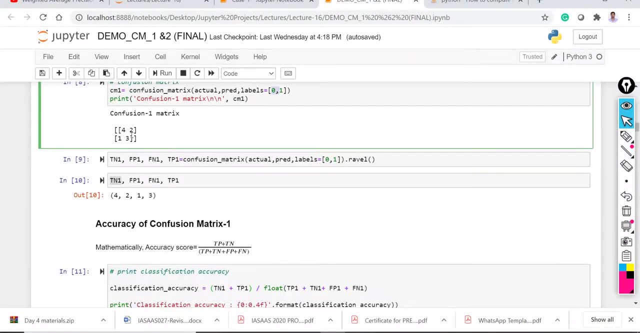 matrix. actually for binary class means there are the two classes, class 0 and class 1, class 0 and class 1, and for class 1. this is the confusion matrix. so based on this values. so here this is a true negative. so what is the meaning of 1? 1 means this is the confusion. 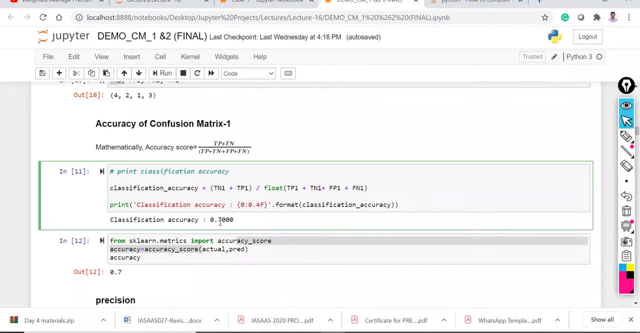 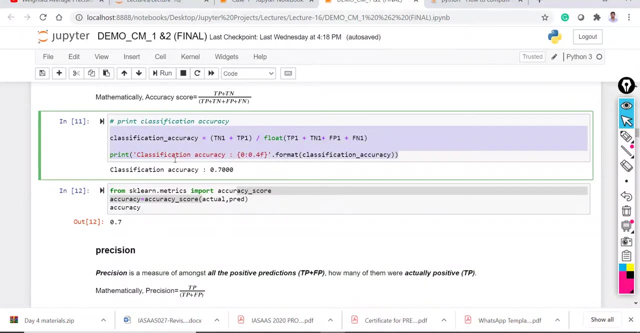 matrix 1. so accuracy of the confusion: matrix is the true negative plus 2 positive by all predicted items. that is the accuracy of the matrix 0.7. so this is the cell number 11. this is the result of the mathematically and cell number 12 is the result of the by coding. so 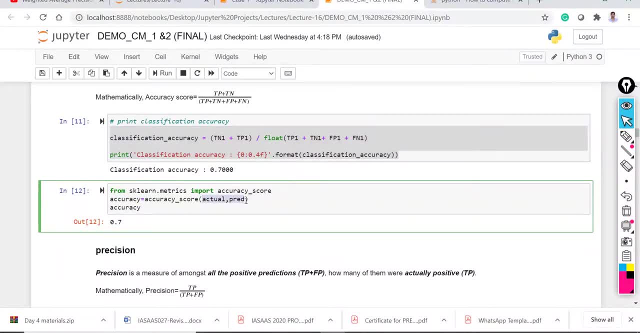 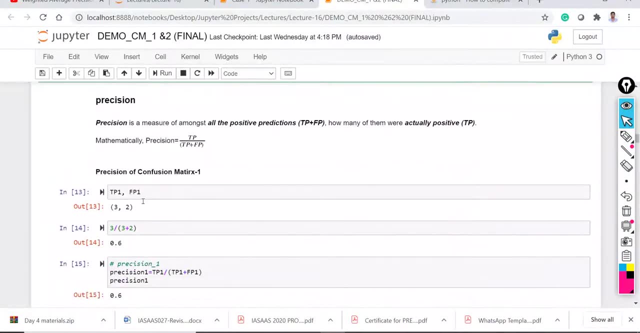 I am applying the accuracy score library on the actual comma predicted. you got the 0.7. so cell number 11, cell number 12, both are getting the accuracy score. so this is the same score. so next evaluation matrix is the precision. so what is mean by precision? precision? 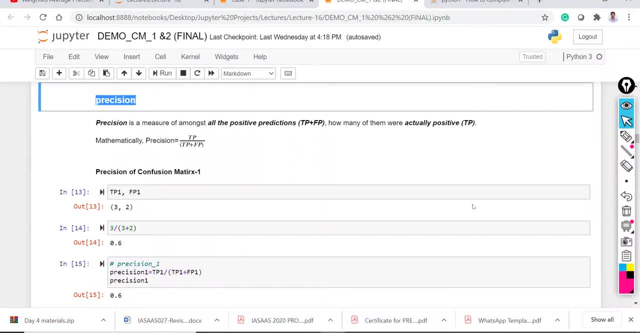 is the measure among the all positive predictions. all positive predictions means so this is the true negative, false positive, true positive and false negative. and y axis. I am considering the actual values here, I am considering the predicted values here: 0, 1, 0, 1. so means precision. 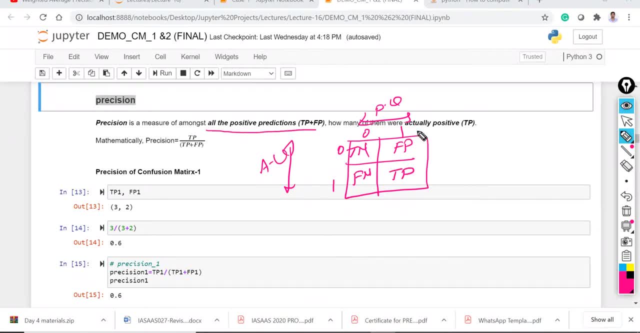 is measured, the all positive predictions. all positive predictions means so this is the all positive predictions by the model. so which means this? this value is the tp plus fp means so this is the all positive predictions given by the model. among the all positive predictions, how much is actually positive? 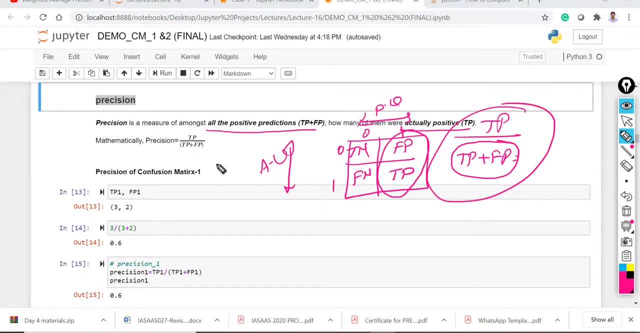 how much actually positive means. this is the tp, so this is the formula of the true positive. so tp by tp plus fp. tp plus fp means this is the out of all positive predictions. this is out of all positive predictions how much we correctly predicted. so this is the precision. 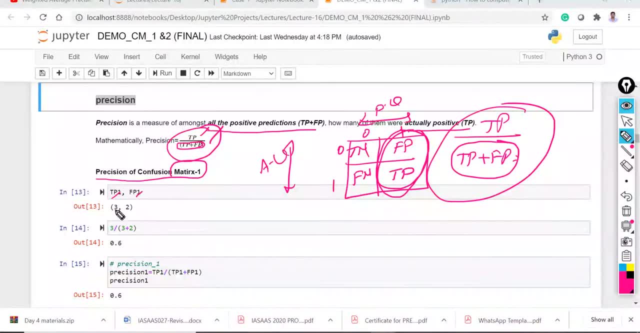 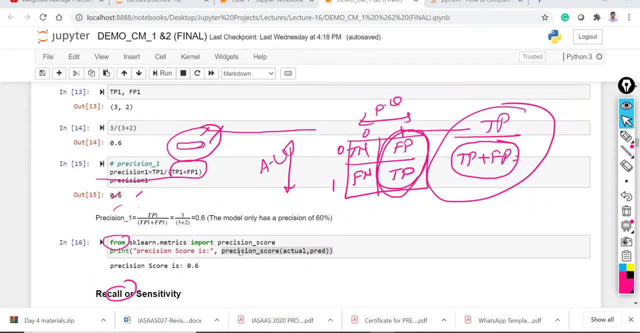 of confusion: matrix 1, so tp 1, fp 1, value 3, comma 2. so if you calculate mathematically 0.6, so by programming also you got the same 0.6. so precision 1 is equal to tp1 by fp1. tp1 means: 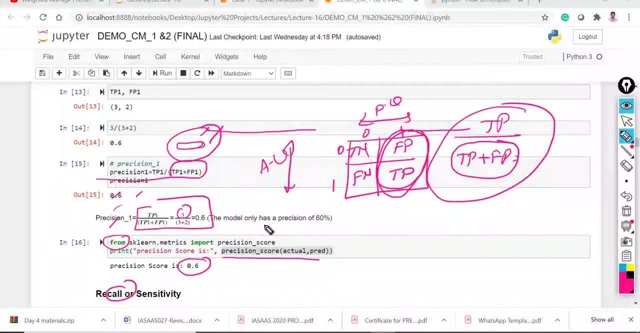 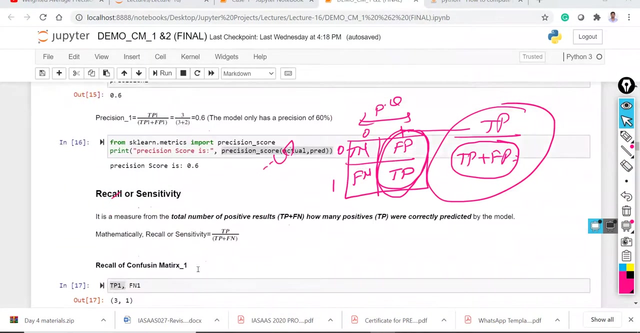 value 3 and 3 plus 2 is equal to 0.6. the model only has the precision about the 60 percent, so this is the about the precision, if you see the recall. so this is the total number of positive predictions, total number of positive results here, not 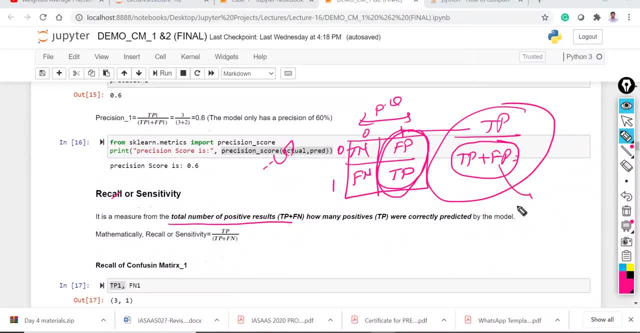 in precision means total number of positive predictions. this is the total number of positive predictions here: total number of positive results. total number of positive results means this is the value. so this is the total number of positive results. so means that this is the tp plus fp. 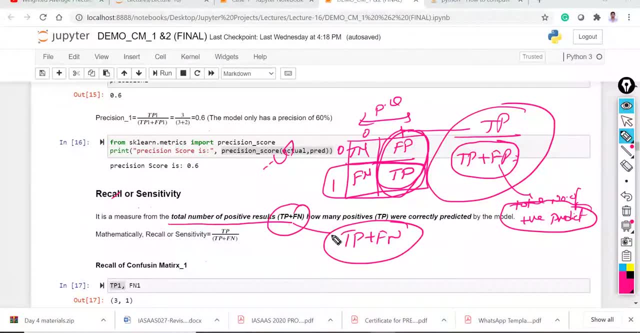 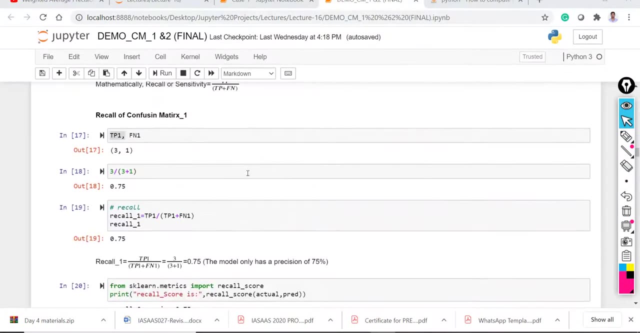 this is the total number of the positive results. out of the total number of positive results, how much? the true positive, which means tp by tp plus fp, means tp by tp plus fn. so this is the formula of the recall. if we execute the cell number 12 as a: 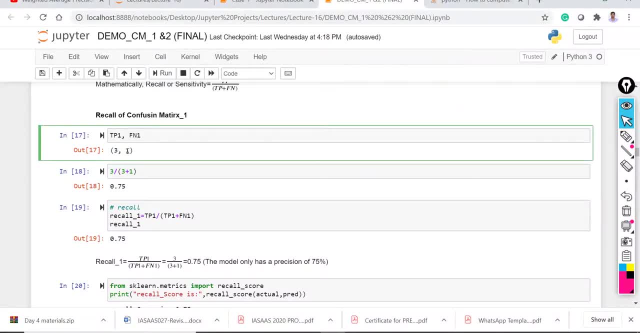 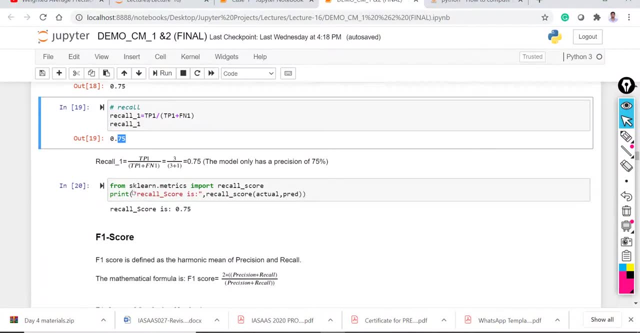 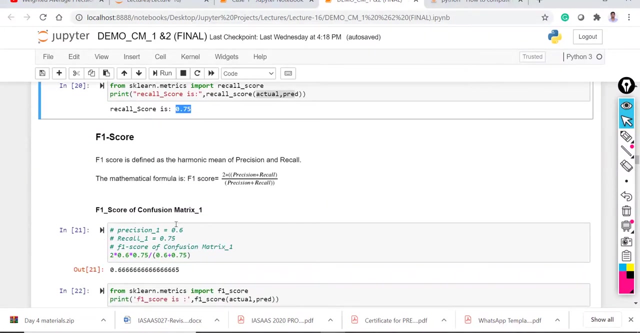 17, the tp1 value 3 and fn value 1. so if you got the 0.75, so by formula you got the 0.75. so by coding in cell number 20 you apply the recall score library on the actual comma predicted. you got the same score, 0.75. so next evaluation metric is the f1 score, so f1 score. 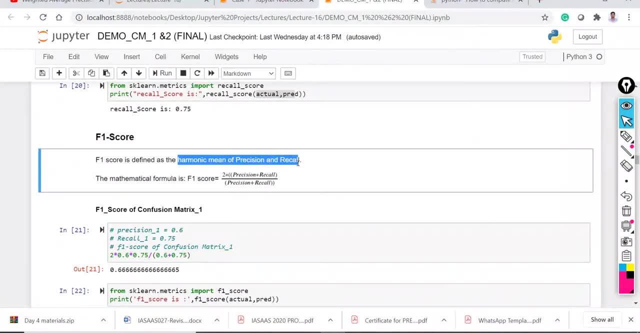 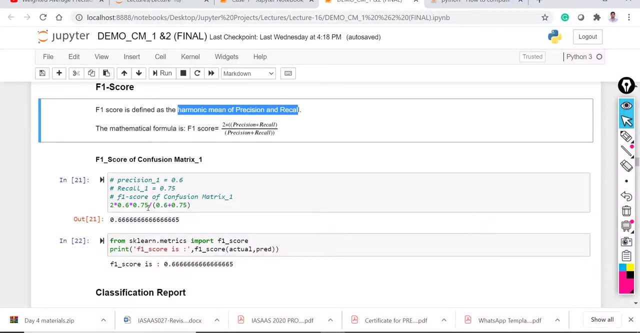 can be defined as the. it is the harmonic mean of the precision and recall. so what is the mathematical formula? 2 into precision, into recall, divided by precision plus recall you. so if you apply this precision and recall of the confusion matrix, so what you supposed to get the f1 score? so precision 1, 0.6, recall 0.75. if you apply on the f1 score, confusion, 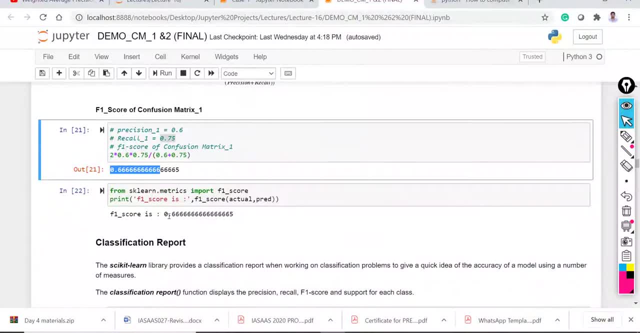 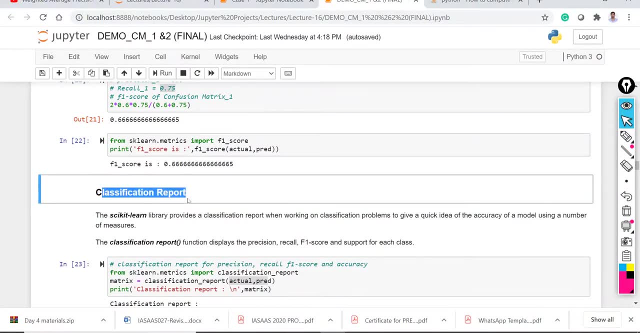 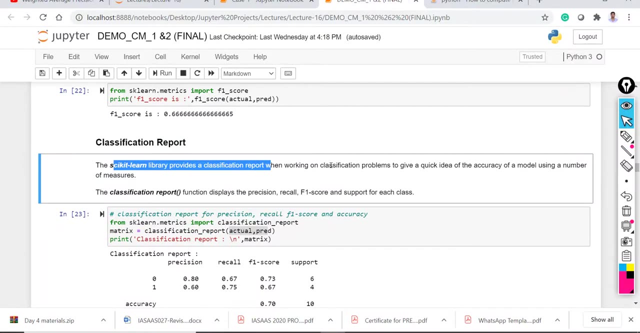 matrix you got the value 0.66, which means it is about to 0.67. so if you so here. next one is the classification report. so what is the classification report here? the cycle is the cycle, see the lap, the here the. so Explore the. 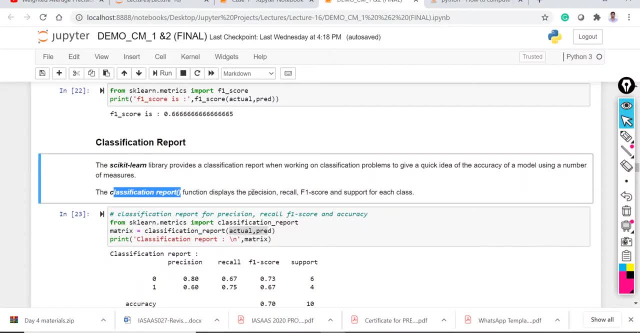 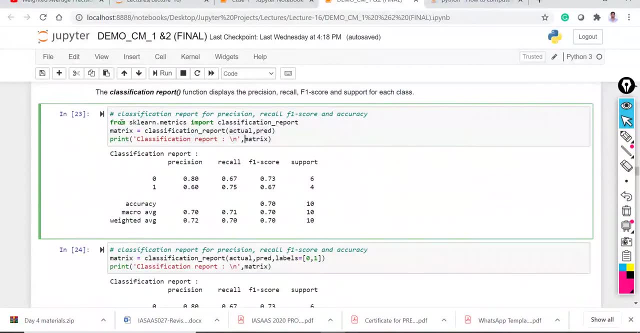 learning sehe, the classification search line الص library. it can display the precision, recall and F1 score and support of each class. so this is the scikit-learn library. from sklearnmatrix you have to import the class. that is the classification report. so from classification report, hball comma. 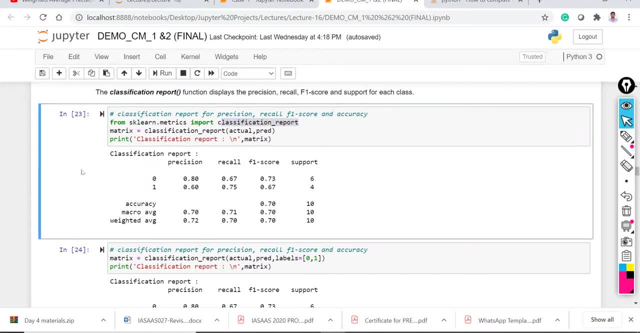 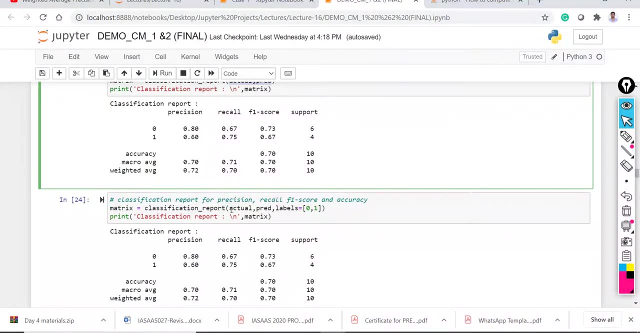 corrected. this is the value you got. so if you observe this, cell number 23 and cell number 24, you both are, the output is the same, but coding little bit difference. so here confuse, and class coefficient report is applied on hball comma predicted, but here, as classification report was applied on hball predicted. 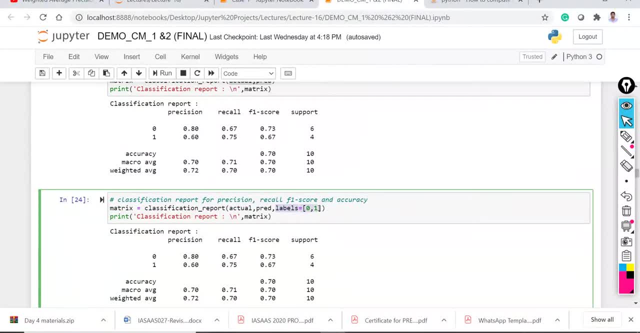 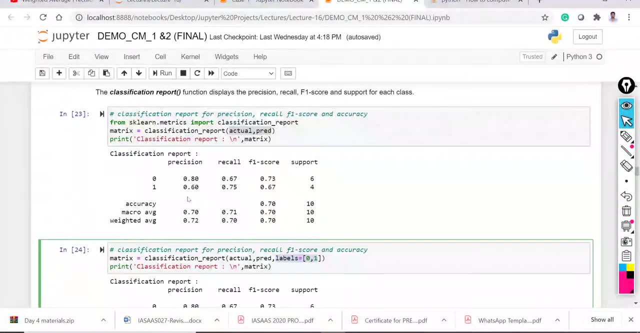 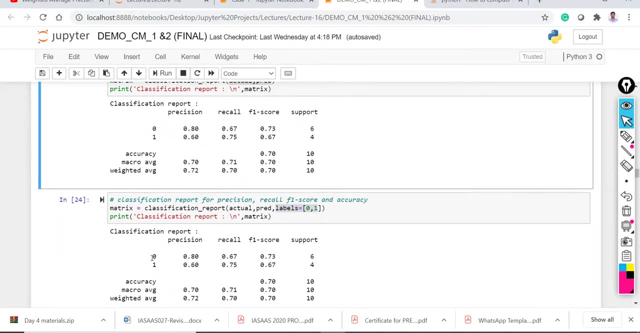 and labels. so here I mentioned the labels, is equal to 0 comma 1. so if you are not able to mention the labels 0 comma 1, so it will display the give the output the same. so no change at all. so here see: first it is 0, 1, here also be. 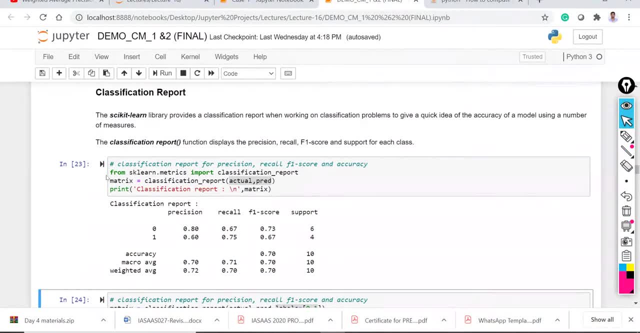 same thing. so in the classification report, if you observe, so this is the precision value got by formal and coding, and this value we got 0.75, 0.64, so for class 1. so here support means how many number of 1, 4. so this is the about one fulfillment. so 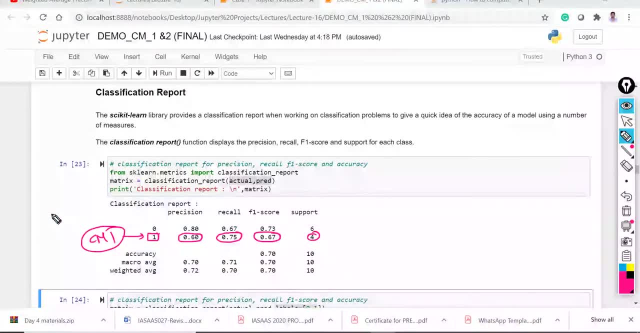 this is the confusion matrix one. so confusion matrix one. given what is the confusion matrix four, two, one, three. so in this confusion matrix, you have to apply the precision. this is the precision value and this is the recall value and this is the f1 score value and total number of ones. total number. 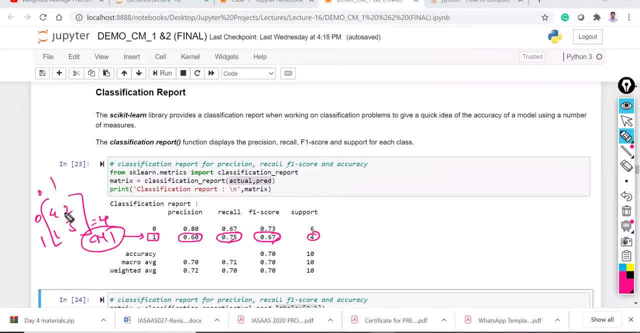 of ones here: four here. total here: zero comma one, zero comma one. here total number of ones is four. total number of zeros is equal to six. so total number of zeros is equal to six. so now we have to calculate this one more confusion matrix. so for class zero, now we calculate the confusion. 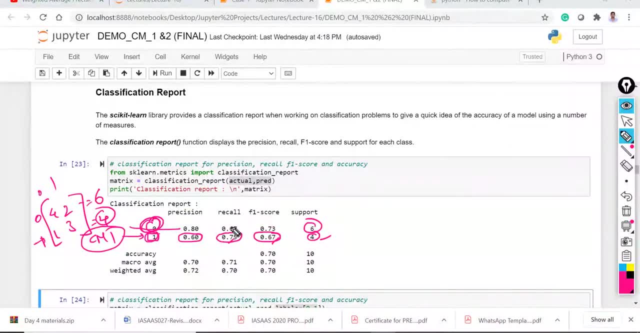 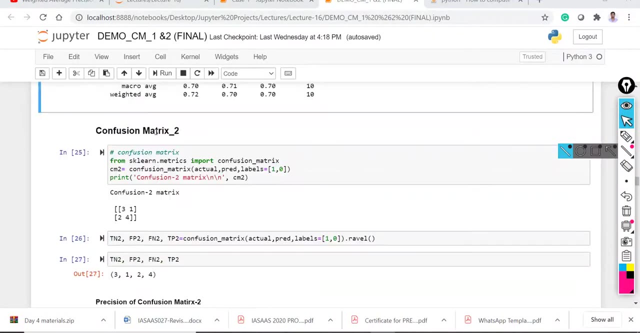 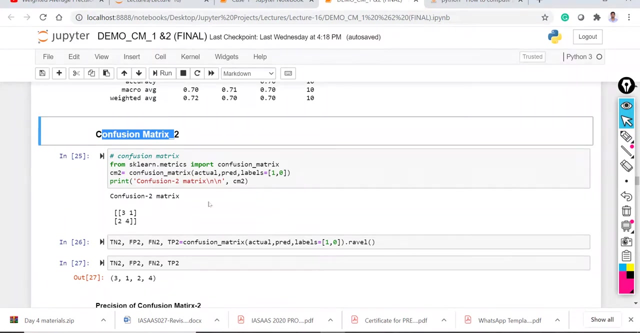 matrix for class one. this is the values we got. so now we have to, we have to find the another confusion matrix. so another confusion matrix, if you see. so this is the confusion matrix two. confusion matrix two means for, if you see the confusion matrix, if you see one comma zero, if you give one comma zero, this 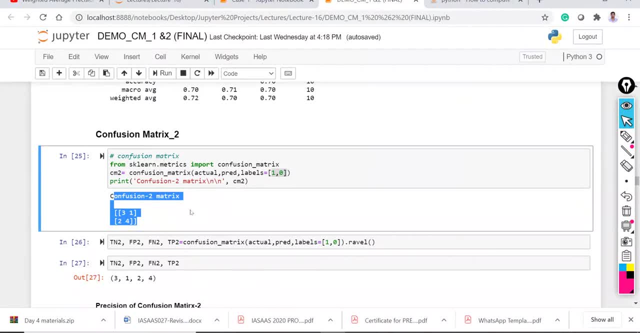 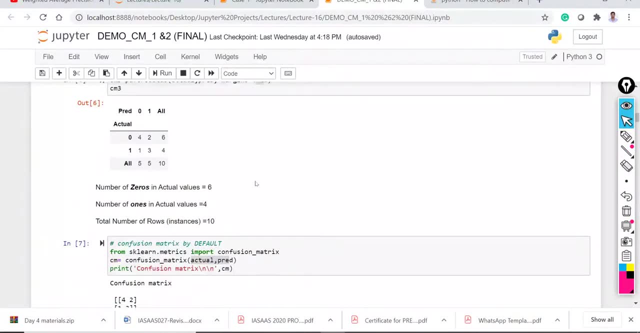 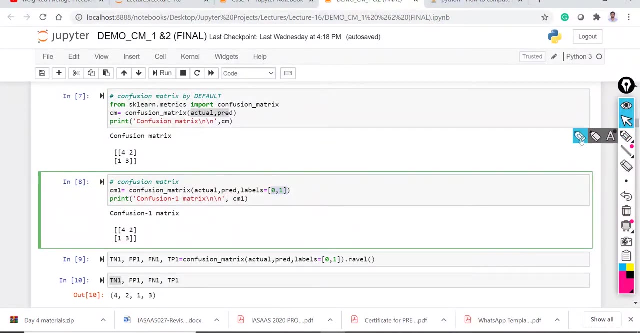 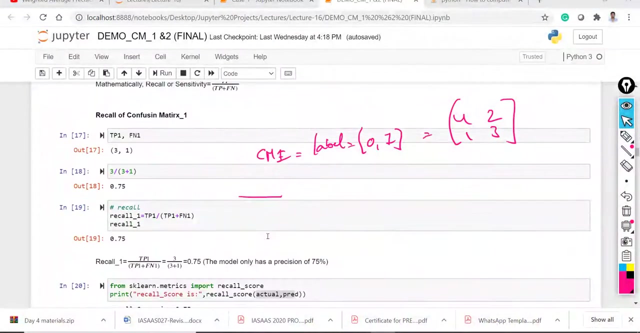 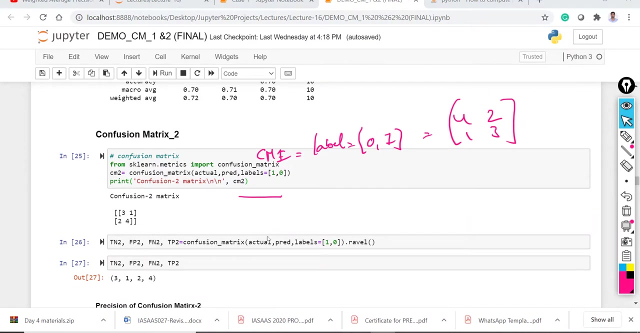 is the matrix. you got confusion matrix three, comma two, if you see the cost here one zero one, here zero one. so confusion matrix one here to labels zero, comma one. you got the four, two, one, three, confusion matrix. if you come here, this is the confusion matrix two. 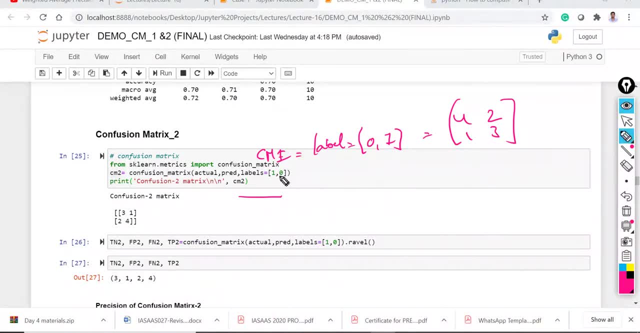 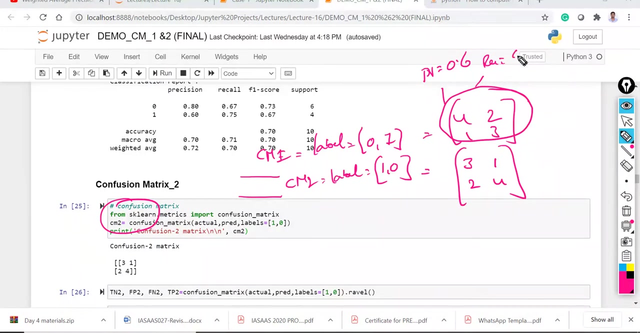 okay, two. so confusion matrix. two means here labels, is equal one comma zero. so what you got? the confusion matrix three. one, two, four. so this is the confusion matrix one. so for this confusion matrix you got the precision point six and recall and recall you got the 0.75 and f1 score 0.67. so these three values suppose, see, this is the. 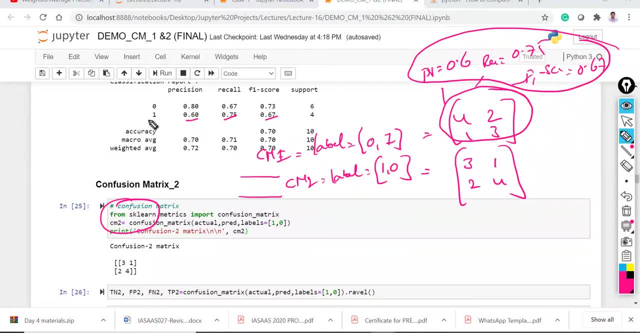 three values: 0.60, 0.75, 0.67 for the confusion matrix one. so here confuse matrix two means labels is 1 comma 0, you got the 3, 1. so from this confusion, matrix 2, you got the precision is equal. 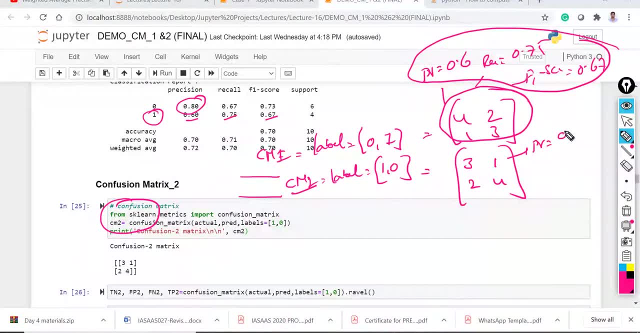 to. so this is the value 0.80, 0.80 and recall 2 is equal to 0.67. so precision 2, precision 1 means confusion, matrix 1, recall 1 and f1 score 1. 1 means confused matrix 1. so here precision 2 means: 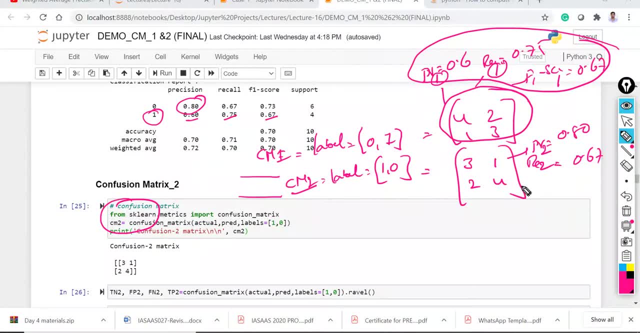 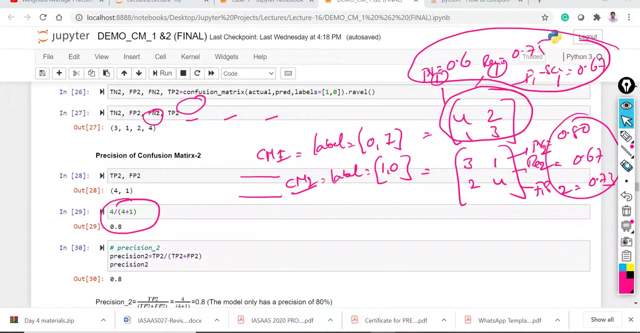 confusion. this is the precision of the confusion. matrix 2. like that: f1 score: 2: 0.73. now we will check these values, how we will get see here: precision of the confusion. matrix 2. so tp value 4. so this is the tp value 4 and fp value 1. you got the 0.8. so this is the 0.8 we got. 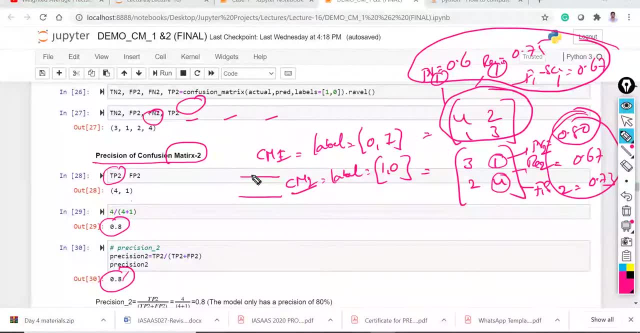 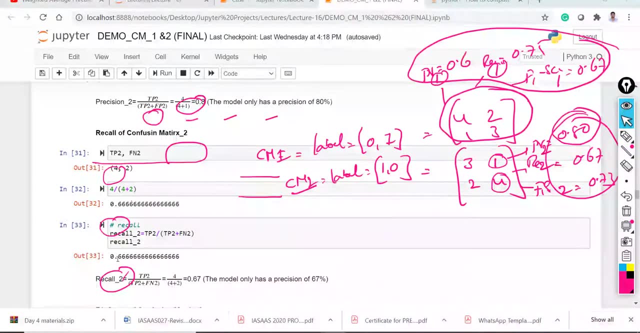 and by formula, because you for by the formula, you got the 0.8, the same thing, and recall you got the 0.667, means it is about to approximately. this value is approximately 0.67. so this is the recall formula, so this is the recall value. 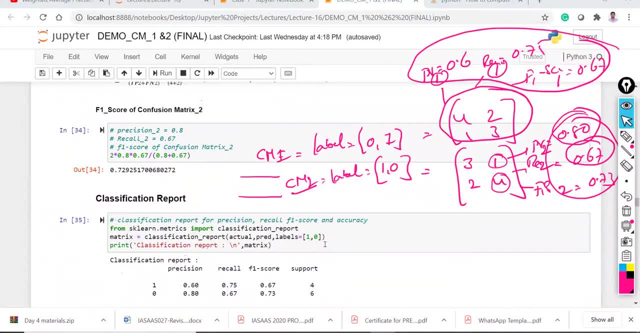 if you apply the f1 score on confusion matrix 2, so f1 score of the confusion matrix 2, the precision is 0.8 and recall is 0.67 and you got the f1 score is 0.7293, which is approximately 0.73, see 0.73, 0.67 and 0.80. so the values we got the same thing. 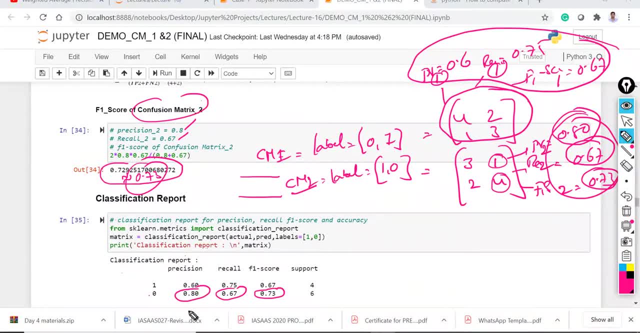 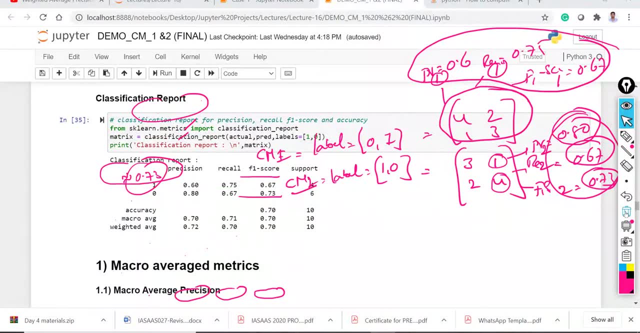 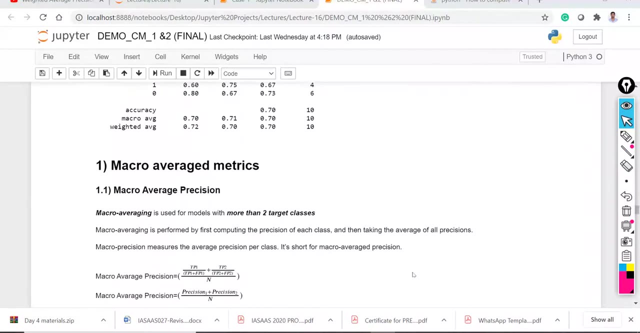 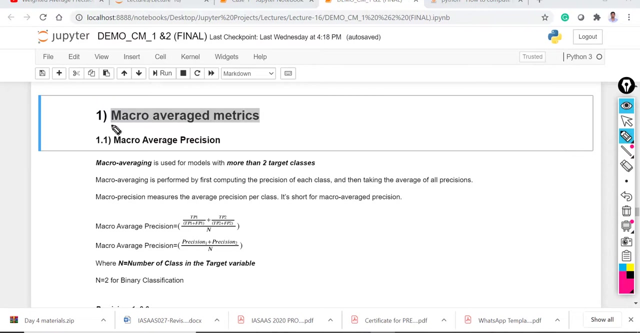